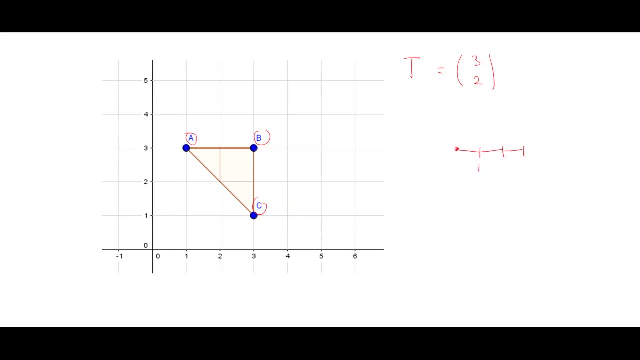 three, three units. So one, two, three units to the right, because it's positive and we're going to move one, two units upwards, right, And this will be our new point. So if we have a point P and it moves to the point P' right, This represents a translation and it is represented. 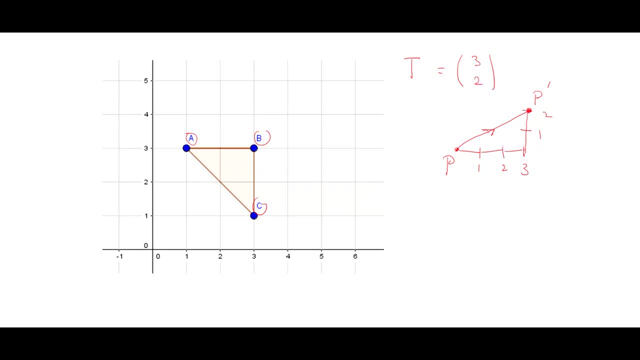 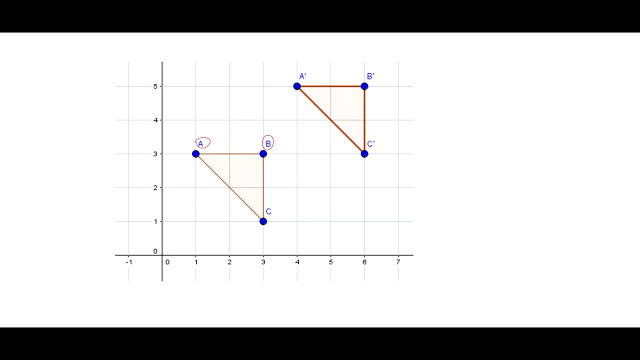 by the column, vector 3, 2,. okay, So let's look at this example here. So we have triangle A, B and C and we undergo a translation T, which is given by division Vector 3, 2.. So if we look at the point A, we have to go three across, So we go one. 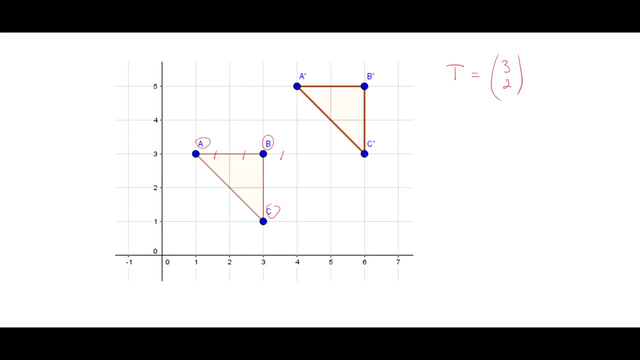 two, three across, and then we're going to move one, two upwards right. So therefore this line here represents the translation of the point A, Then we're going to do the same thing with B, So we're going to go one, two, three, three, four, five, six, seven. eight nine, 10,, 11,, 12,, 13,, 14,, 15,, 16,, 17,, 18,, 29,, 30,, 31,, 32,, 43,, 43,, 44,, 45,, 46,, 47,. 50,, 41,, 42,, 45,, 48,, 42,, 44,, 45,, 47,, 51,, 42,, 43.. You get the answer between column B, then column C. It's one, two, three, and then we're going to go one, two up. So therefore, B will. 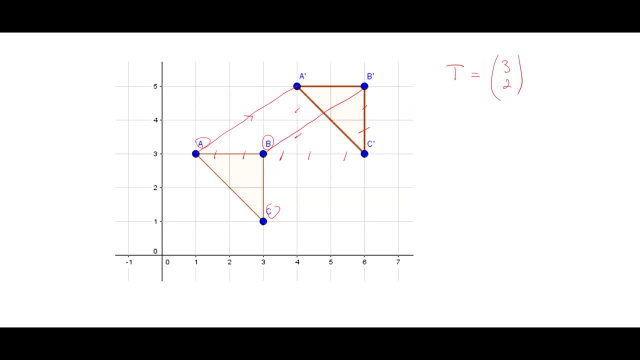 move to this point here, right. And in the case of C, we go one, two, three across and then one, two upwards. So therefore now this represents, because I just showed you the front of the three points- we move one to this point here. The second, isėp**oミ. 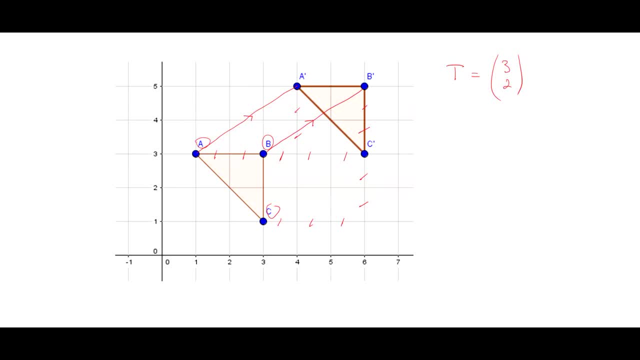 nə two. If this was actual, then I'd still be saying that this is the same one, two upwards. so therefore, now, this represents the object that is undergoing the transformation and this represents the image. now, what can we say about the object and image? now, the object: the lengths are identical to the image, and 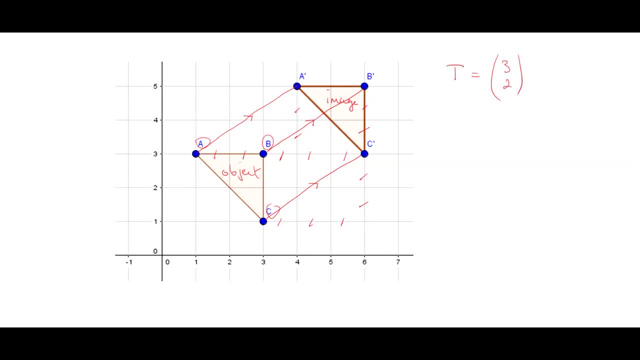 the orientation of the object and image are the same right. so what? we see that the object and image are congruent. all right, this is a term that they expect that you see when they ask you to compare an object and an image, when it undergoes that translation right, the object and the image are congruent, meaning that they have. 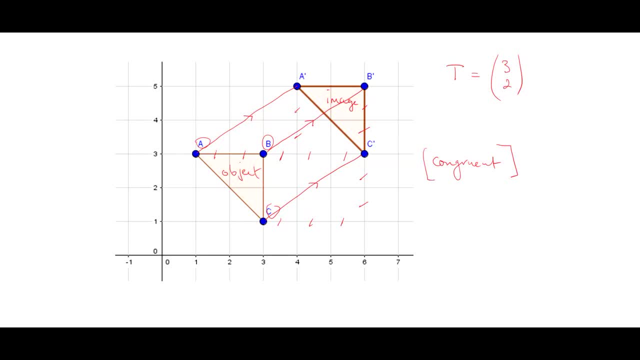 the same lengths and the angles in their triangles are the same. okay, now if you notice the line joining a, a prime, b, b prime and c- c prime, they're all parallel, right, meaning that each point on the triangle is translated using the same column vector, which is three, two in this case, right? 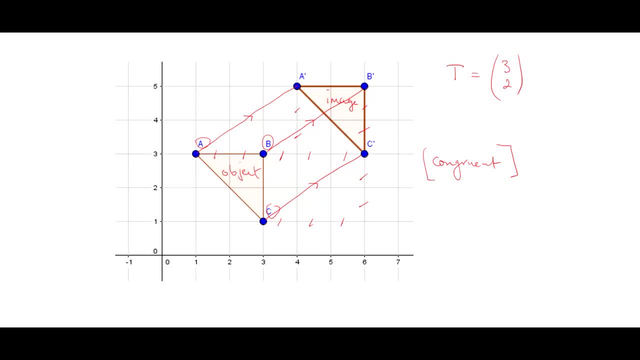 now a typical examination question. they will give you a diagram and they may give you the object and the image- and asks you to describe the transformation as fully as you can. so, because we know that we have a triangle here, the object, and we're moving to this new position which 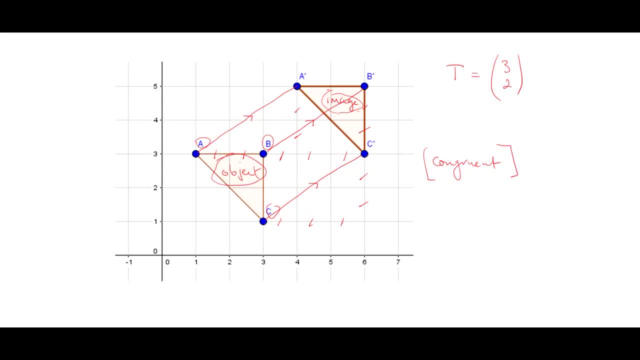 which becomes the image using a translation given by this column vector here, which is 3, 2.. Now in the multiple choice exam you may see a question that looks like they will give you the coordinate of one point. So let's say the coordinate of A is 1, 3.. 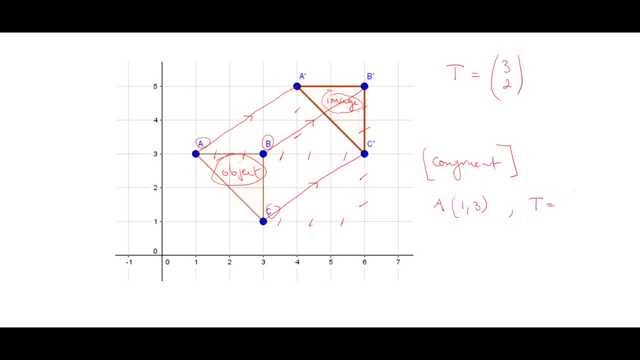 And they come and they tell you that the translation is given by 3, 2.. Determine A'. In order to do that, we write A as a column vector, which is 1, 3. And we add it to the translation, which is 3, 2.. 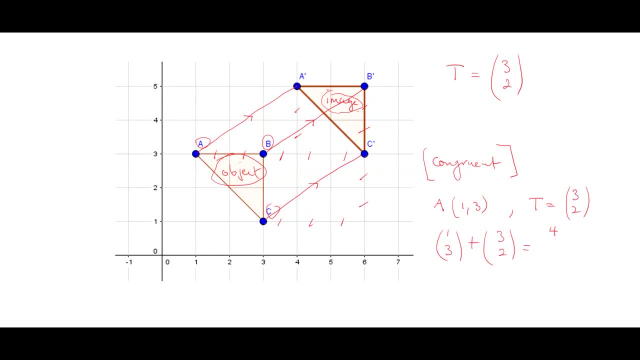 And we get 4, 5.. So the coordinates of A' is given by 4, 5. And we can check that here. What is the coordinates of A' What is the coordinates of A' If we come down here? we get 4, 5.. 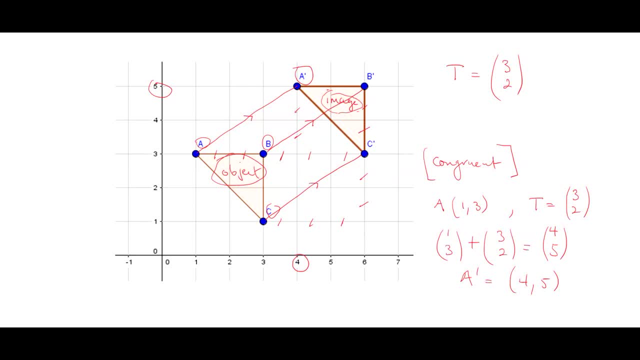 Right, So you can read it off directly from the graph or you can calculate it. So this is typically what you might see in a multiple choice exam In an essay type or the paper 2, you might see. it might give you a diagram and it asks to describe the transformation. 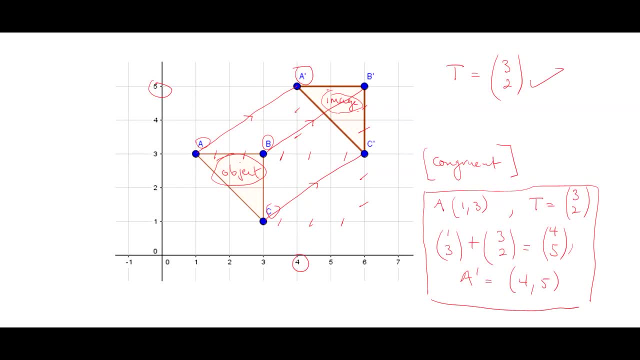 Right. So you must provide the column vector in this case And if they ask, they must provide the column vector. If they ask you to compare the object and the image, you need to say that they are congruent, Right? Let's look at another example. 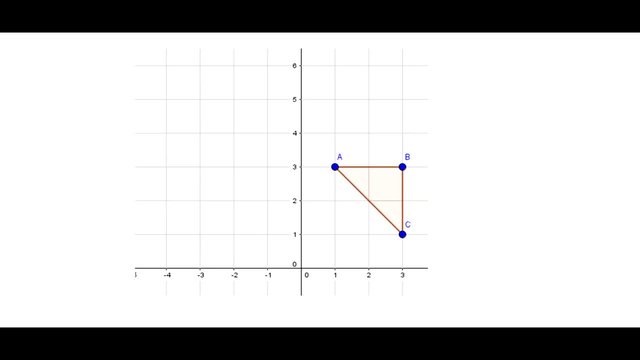 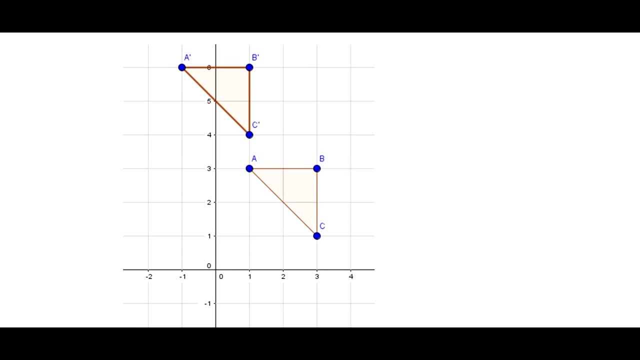 So we have triangle ABC, again Right, And it is undergoing a transformation here. So we have our object Right, And our image. Now let's see what's happening to A and A' C and C' And B and B'. 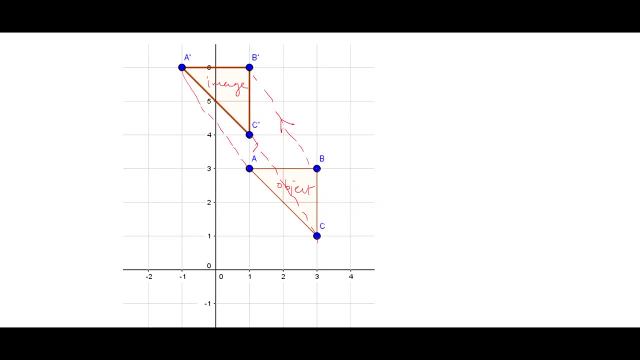 Right. So this is the direction in which we are moving. If it's a translation Right, In the case of A, we are moving 1, 2 to the left Right. So therefore, if the translation is represented by T, 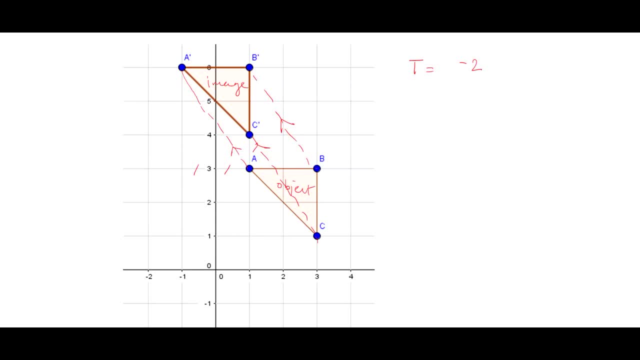 it will be minus 2.. Because we are moving to the left And we are moving 1,, 2, 3 upwards, So it's minus 2, 3.. Okay, Now we can check it with C. Let's say we check it with C as well. 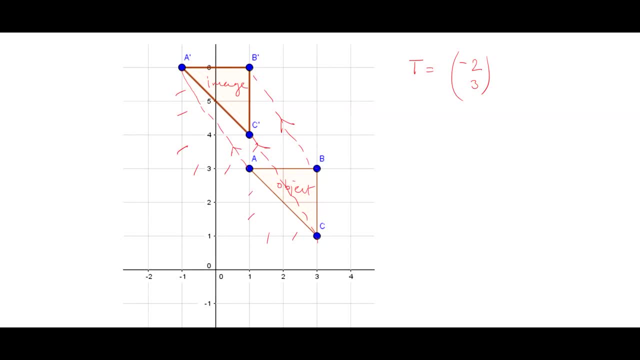 1, 2 to the left, And we go 1,, 2, 3. Up, Okay, And the same thing for B. So this diagram represents a translation which is given by T, And the translation is given by the column vector minus 2, 3.. 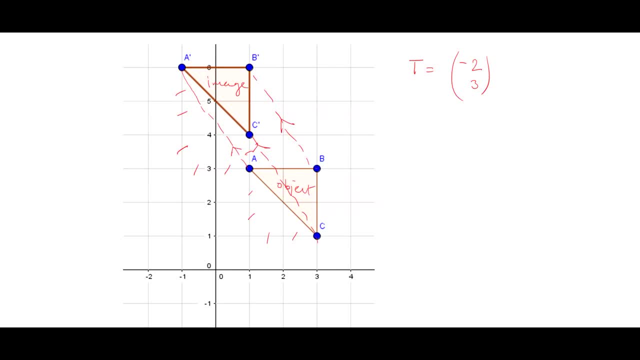 So let me show you something one time In terms of movement: if we are moving to the right, it is positive. If we move to the left, it is negative, And that represents that's in the X direction: Right If we move up. 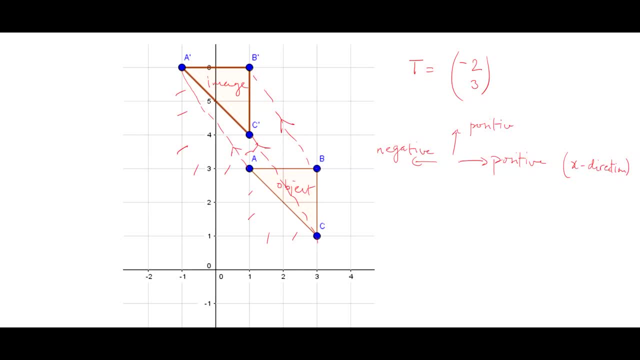 it's positive And if we move down, it's negative. Right, And that we are speaking about the Y direction. All right, In terms of the column vector, the value on top represents the X direction And the number at the bottom represents the Y direction. 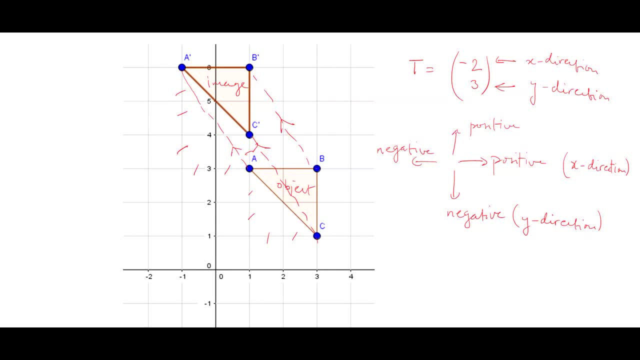 All right. So if we look at C, we would have moved 1, 2 to the left. So we move. so therefore it has to be negative 2.. That's why we got the negative 2 here. then we moved one, two, three in the positive direction. so therefore it has. 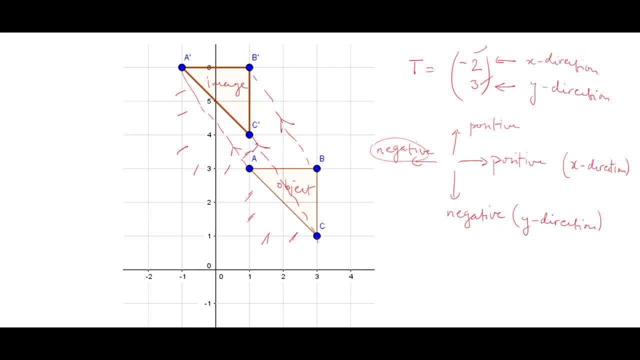 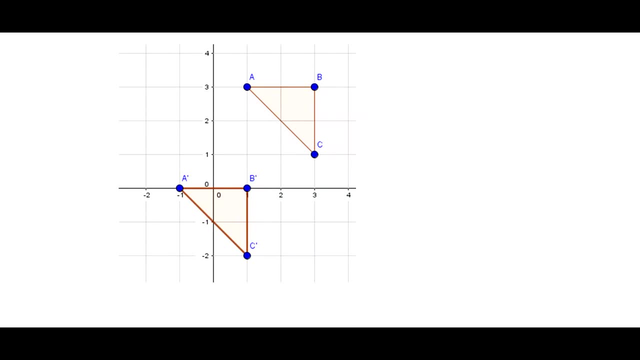 to be three, okay, so let's look at another example here. so we have triangle ABC again. so this is our object and this is our image. and typical examination question: describe the transformation. so if you notice, the object and the image is same size, the same shape. so the idea for congruent and if we look at what is, 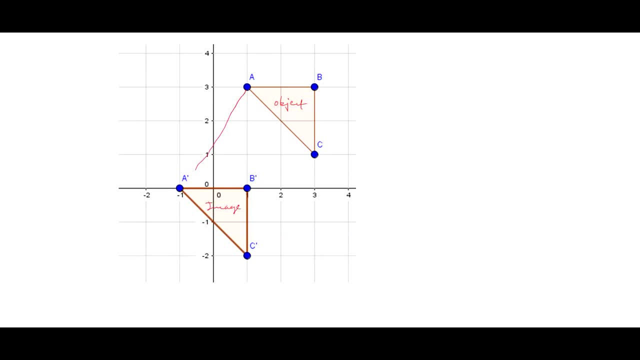 happening to you. he is coming to a prime like this and we are moving one, two to the left, so the translation will be minus two because we moved into the left. I'm moving one, two, three downwards right, so if you're moving downwards, then that is negative. so the translation is given by minus two, minus three. look at what is. 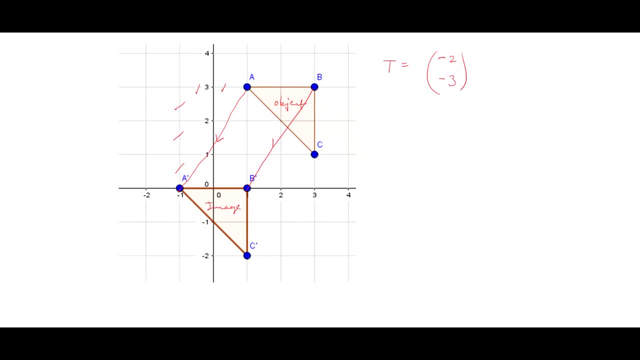 happening to B and C. in case of B, we are doing one, two to the left, so it's minus two, and one, two, three down, so it's minus three. so every point of the object undergoes the same translation. okay, so if we are given A, the coordinates of A is given.